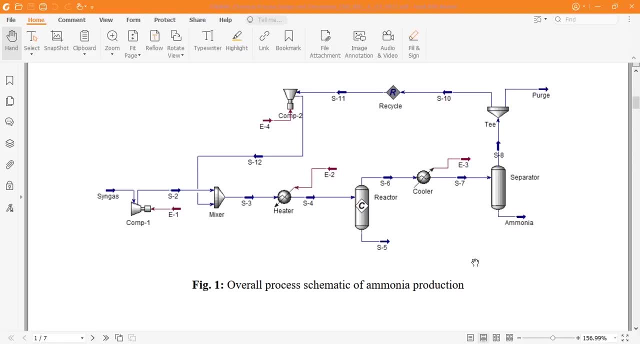 hysis, and this is the overall schematic of the production and, as you can see, the syngas. it is first compressed using a compressor, one to which electricity is supplied, work is supplied, and the compressed stream is then passed through the mixer. I will talk about the recycling portion later, but first discuss this. 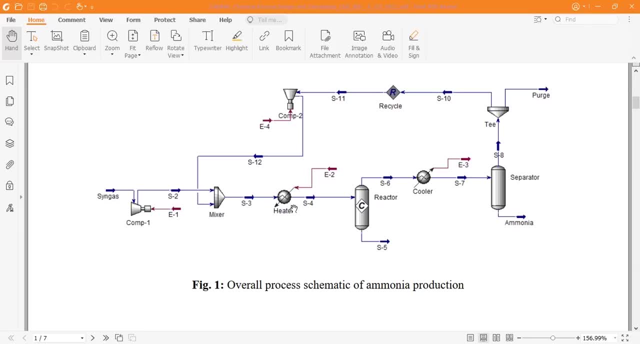 overall scheme: Syngas: first compressed, then pass through the heater, then sent to the conversion reactor, then it is cooled down and followed by the separation. Ammonia is obtained from the bottom of the separator, while the top stream, or the vapor stream, which contains fraction of nitrogen. 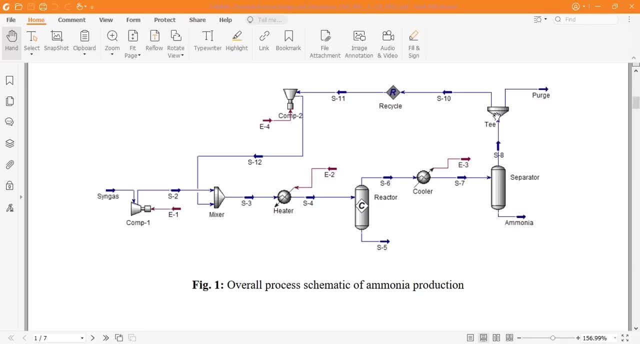 hydrogen and other components in the feed. part of it is purged when the remaining portion is recycled, and once recycled it is again compressed to meet the required pressure of the system and then it is recycled back. So this one, this portion, is the recycling portion. so we will be doing the simulation in aspen hysis. So first, 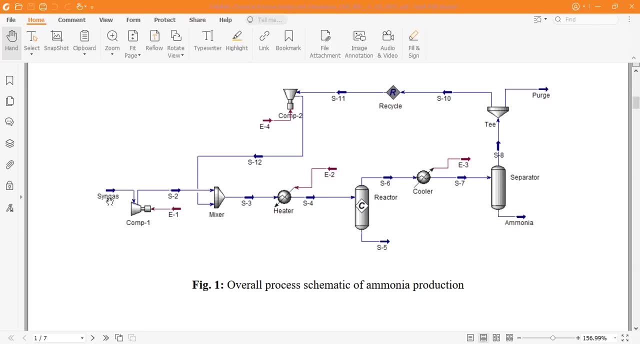 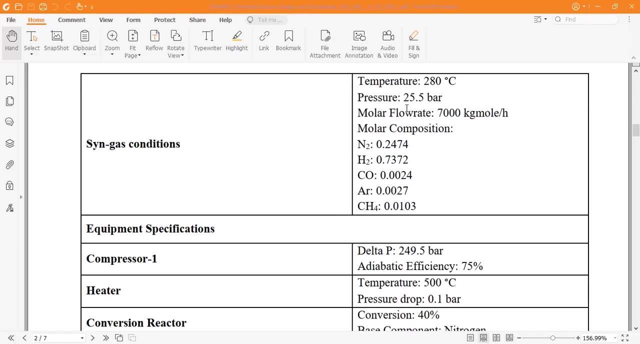 we will build the simulation, then we will give the specifications of feed equipment, so on. so let's quickly move to aspen isis, but first we will read the conditions of the syngas, which is the feed stream, because you know we need to first specify the components. 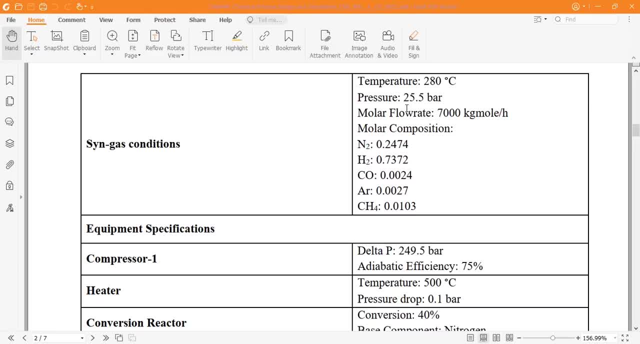 and without specifying component and fluid package we cannot go to the simulation environment. so the component involved nitrogen hydrogen, co argon and methane, and for the ammonia system, obviously we will add a component of ammonia as well and for this system we will be using pang robinson as the property package. so, as you can see, the components are. 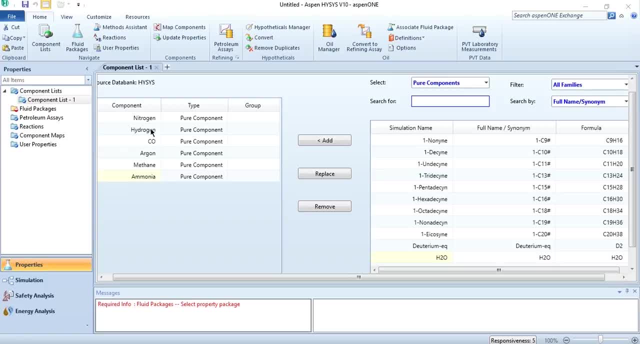 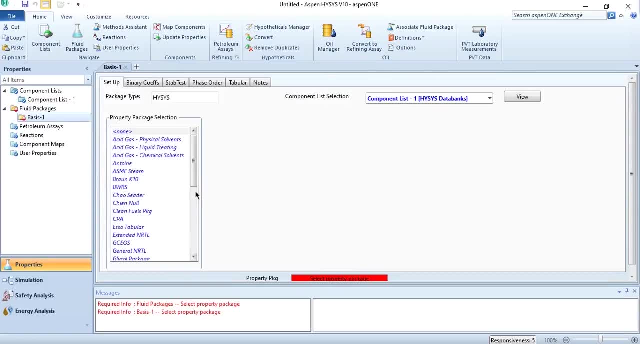 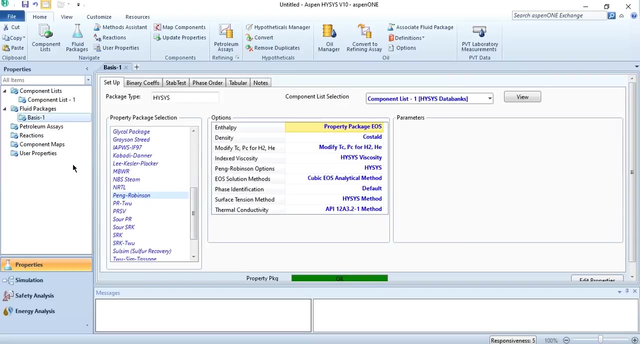 added nitrogen hydrogen. obviously these two are main components. co argon, methane are part of it and ammonia is your final product and in fluid package we will select the fluid package as pang robinson and, as you know, this system involves reactions and, unlike aspen plus in this unit to 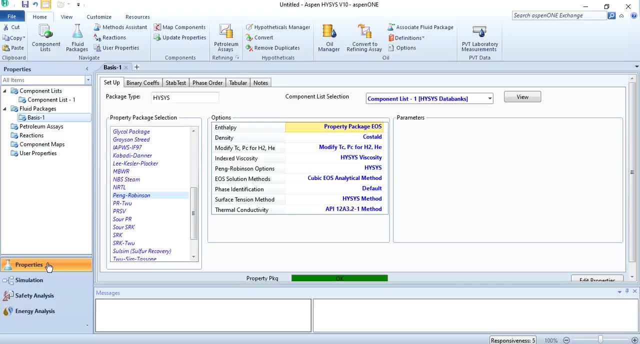 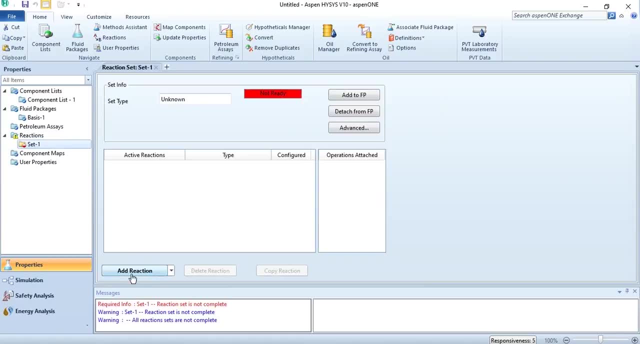 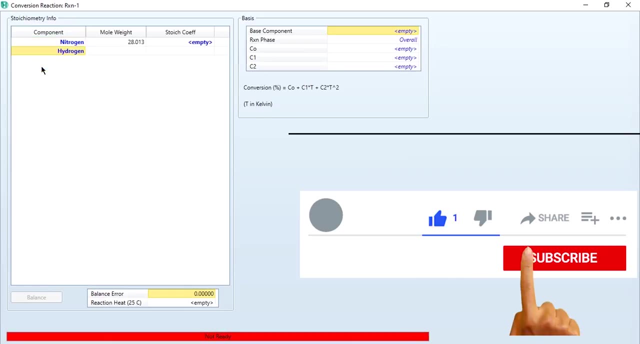 specify reactions in the properties environment. while in aspen plus you will get the components, in s plus you need to specify in the simulation environment, click reactions and what type of vector it was involved: conversion reactor. so we will add the conversion reaction- nitrogen hydrogen and ammonia. and we know minus one, minus four reactant and positive for product: minus three. 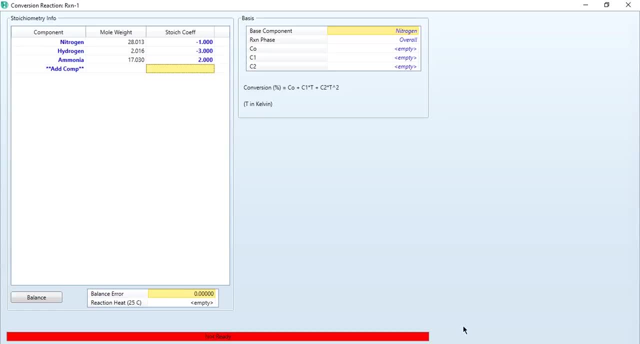 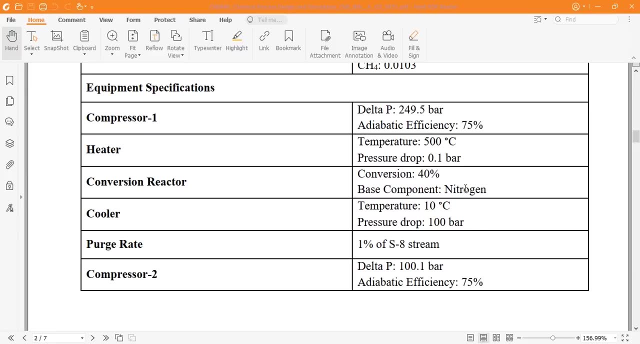 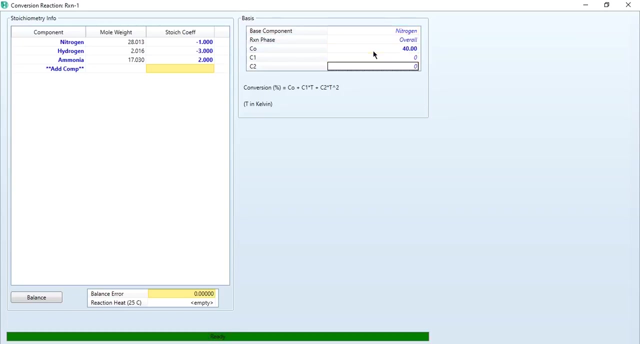 and two and you can see balance. error is zero. if i take you back again, for the conversion reactor, the conversion is 40 percent and base component is nitrogen. so the base component is nitrogen, reaction phases, overall conversion is 40 percent, meaning will be zero. and then you need to attach. 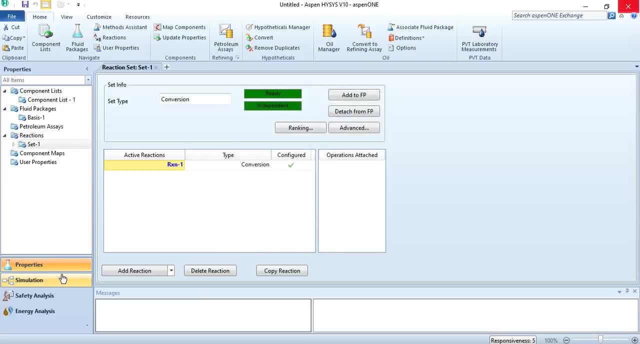 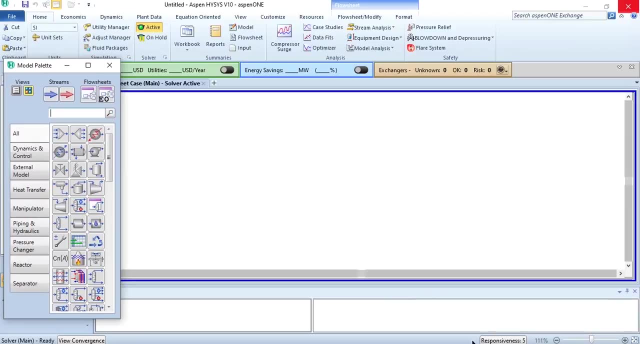 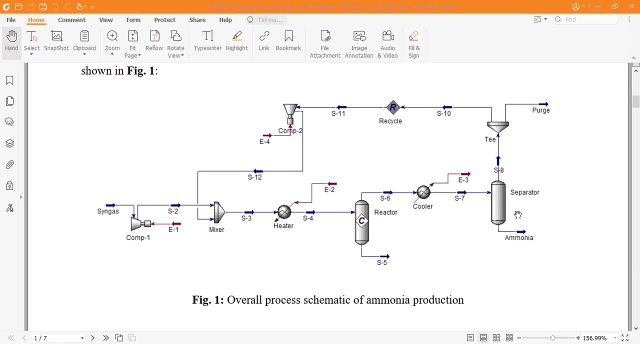 it to third package or add it to fluid package and then you can please proceed to the simulation environment. now, if you look at the diagram again, what are the components which are involved? compressor, mixer, heater, reactor, cooler, separator. so first we will add- so these are the equipments which are added over here- compressor, mixer, heater. 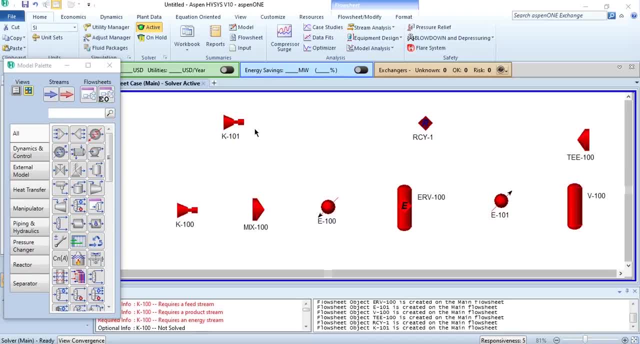 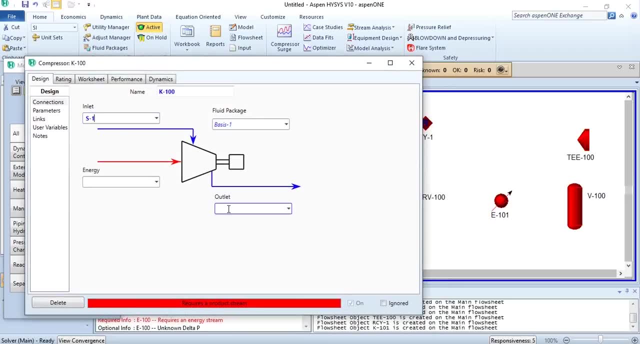 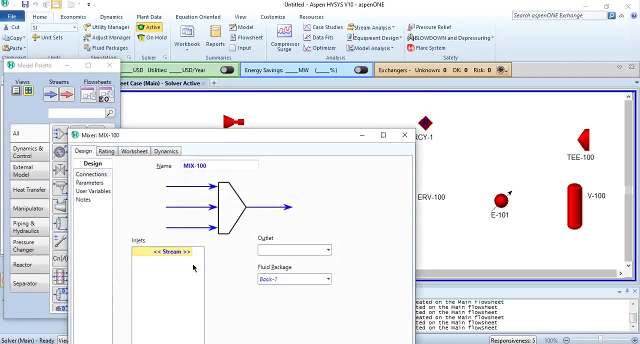 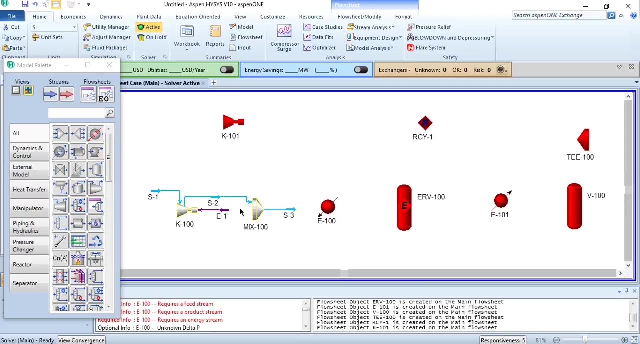 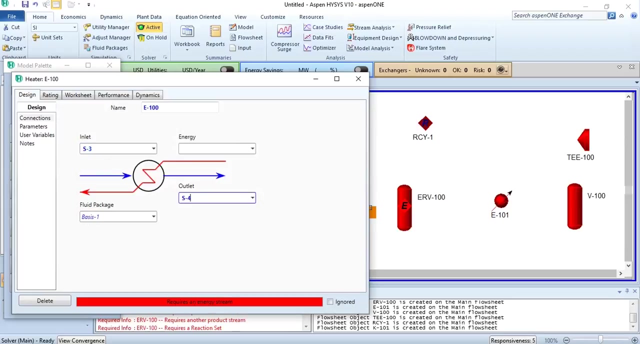 reactor, cooler, separator, t recycle and final compressor. so we will do the connections one by one. this one is s1 and s2 and this one is e1, then mixer, firstly s2 and then s3. we will add the this stream later and i will align it one by one as well. then s3, s4 and e2. 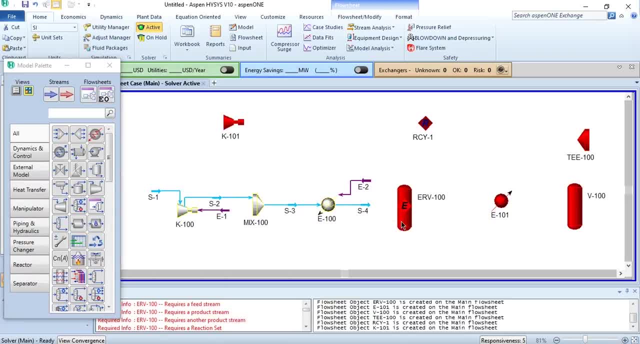 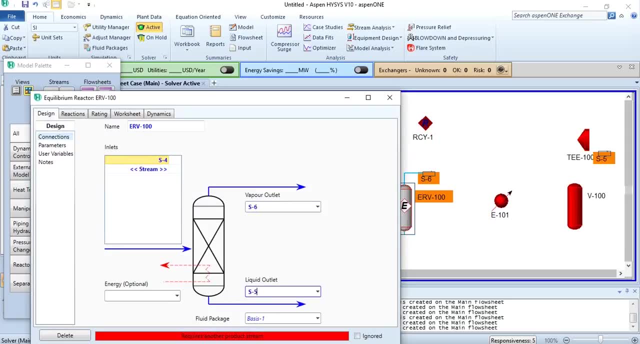 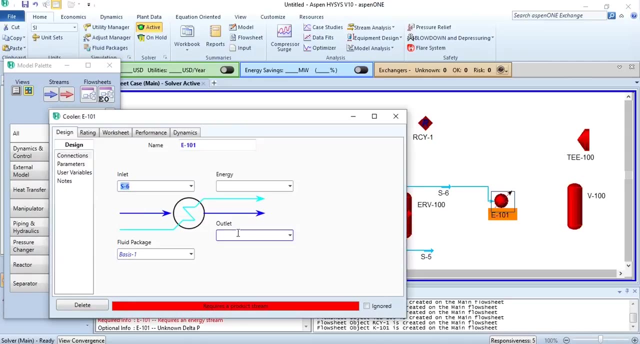 and again a bit aligned so that the flow should look much better. then s4 is entered over here. s6 is vapor, s5 is liquid. obviously it's a vapor phase section, so no liquid will be produced. but you have to show. then s6, send to the cooler, s7- again align it and your pft should look. 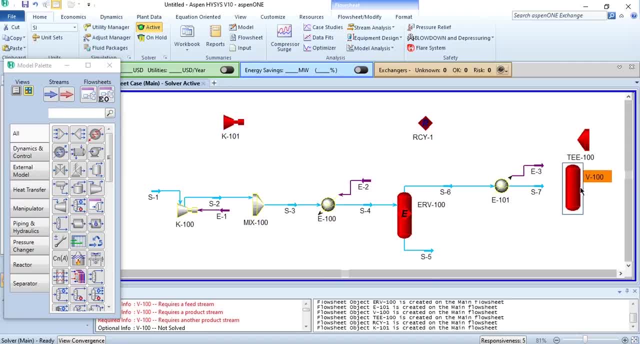 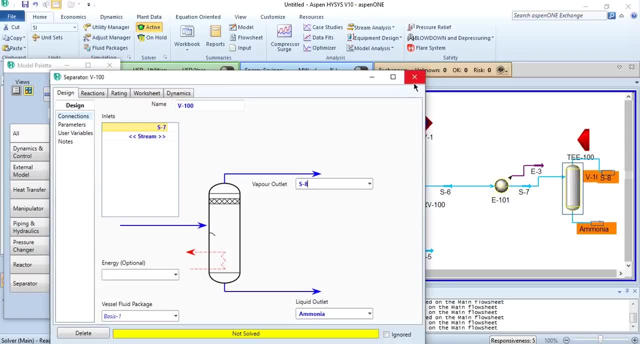 in a much better way for a good representation. then s7, bottom product is ammonia, top product is s8, stream. so first we will solve it and then we will go to the recycle. so what are the specifications? the temperature of the illustrator is 165 celsi. so what are the specifications? the temperature of the 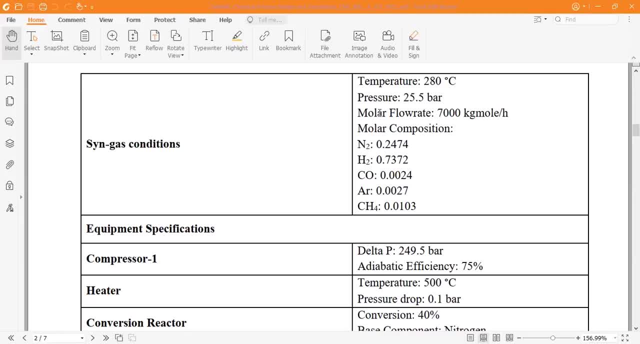 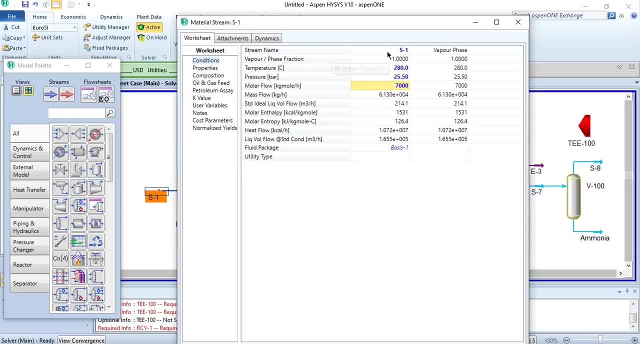 the syngas is 280 degree centigrade, the pressure is 25.5 bar, the molar flow rate is 7000 kg mole per hour and the molar composition is for nitrogen, hydrogen, co argon and methane. so we will enter these in s1 ices. so, as you can see, the specifications are entered of s1. i can label it. 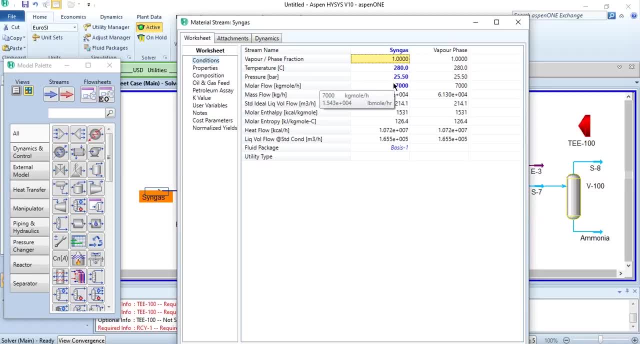 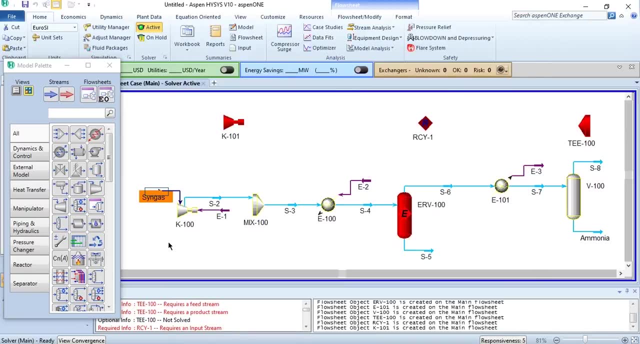 as syngas: 280 degree centigrade, 25.5 bar, 7000 kg mole per hour, and the mole fraction is given over here. and then, what are the specifications of this compressor k1? that the delta p is 249.5 bar. 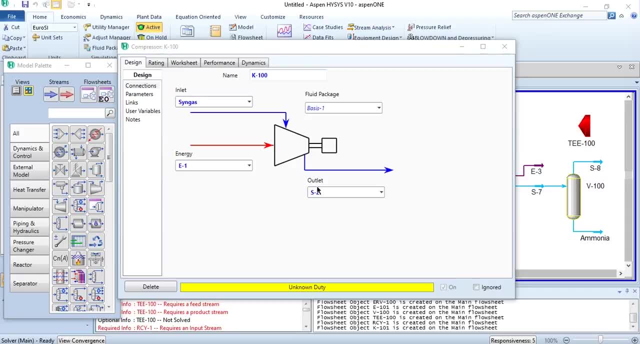 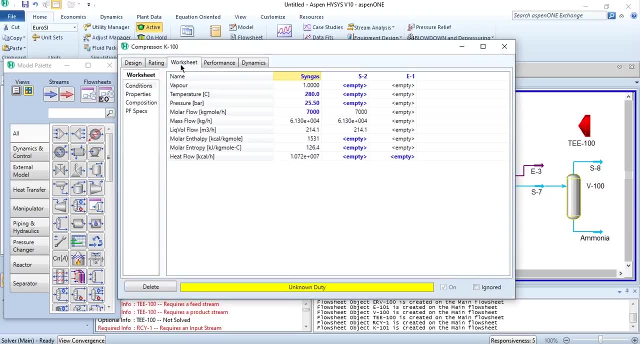 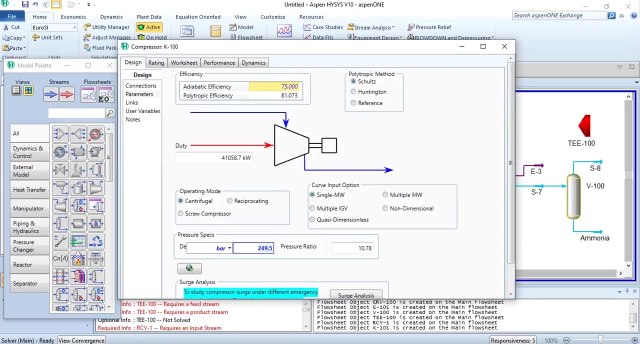 and adiabatic efficiency is 75 percent. if you look at the compressor and go to these parameters you can see this delta p you can specify here. usually in our previous exercises we have specified either outlet pressure or duty. but this is another way of specifying for compressor. 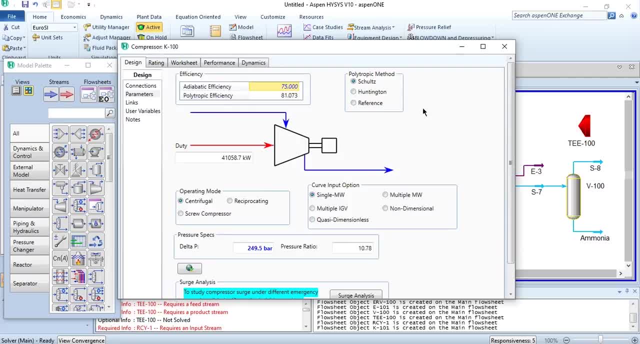 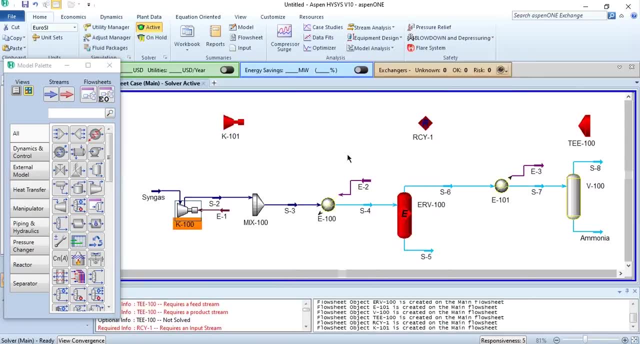 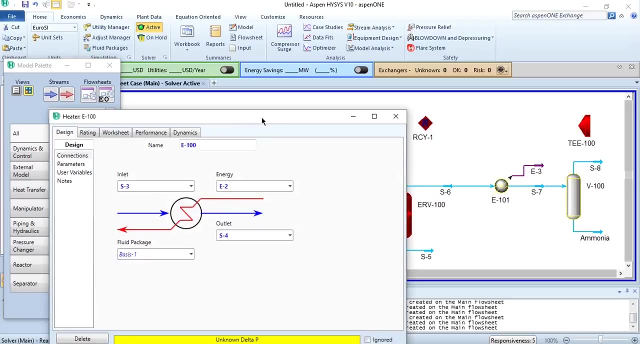 and then adiabatic efficiency is already 75 percent default and, as you can see, it required one parameter because its degree of freedom is one. and you can see, compressor is solved, mixer is obviously solved because there is one inlet and one outlet. then we will go to this meter and its specifications. temperature of 500 degree centigrade. 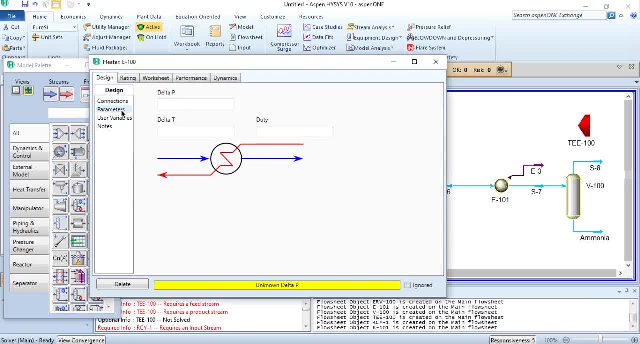 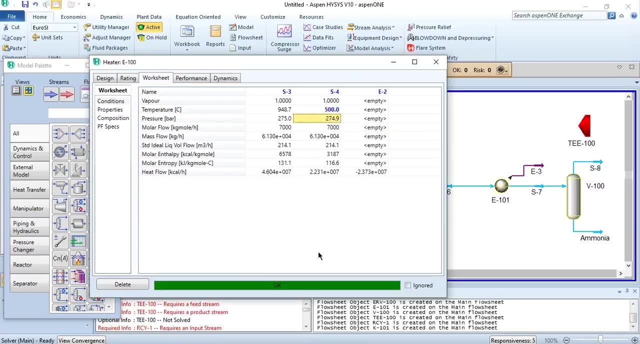 and pressure drop of 0.1 bar. so pressure drop, we can easily specify delta p of 0.1 bar and final temperature as 500. as you can see, its degree of freedom is two. you have to specify temperature, pressure due to temperature of the compressor and, as you can see, it is 500 degree centigrade. and 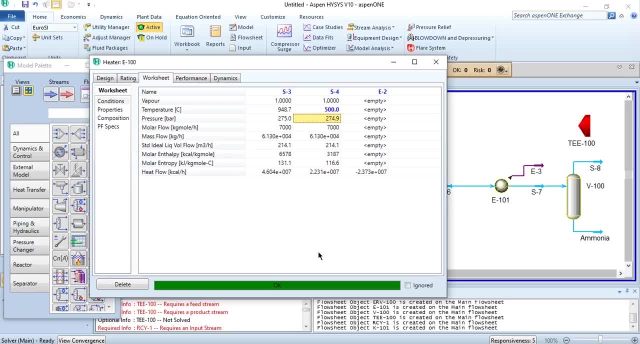 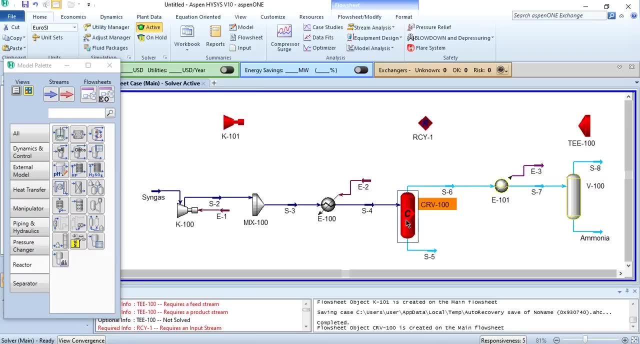 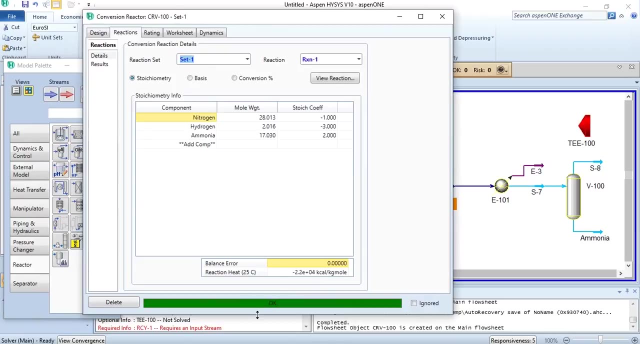 we have specified temperature and again pressure in terms of delta. so we will now go to the reactor- this is conversion reactor- and then we will specify the reaction set and, as you can see, it is okay. results: the conversion is 40 percent and, as you can see, there is no liquid produced and 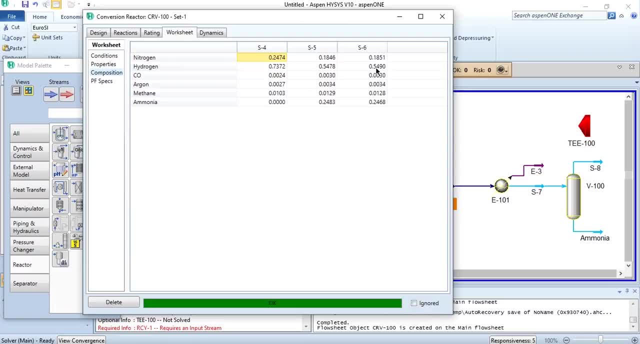 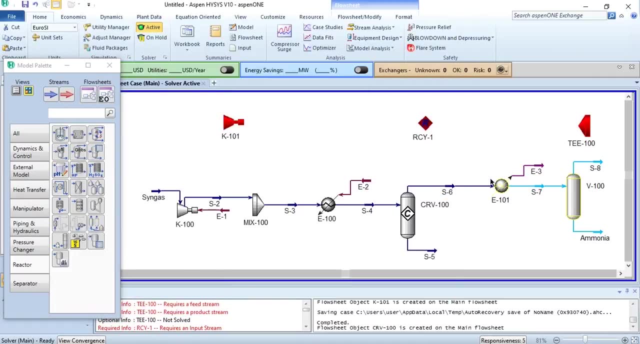 in composition you can see that nitrogen and hydrogen are converted to ammonia, because here in s4 there was no ammonia and now ammonia is present in the system. so now you will go to this. cooler now. and what are the specifications of the cooler? outlet temperature is 10 degree centigrade. 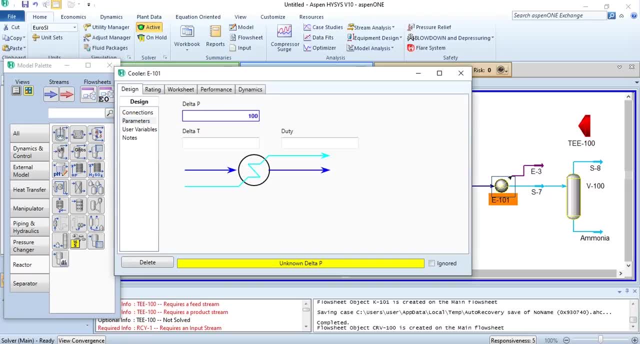 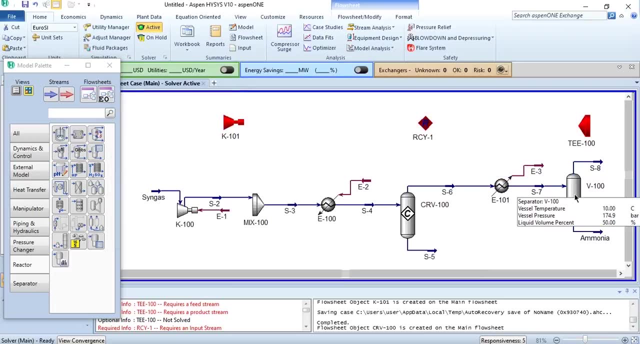 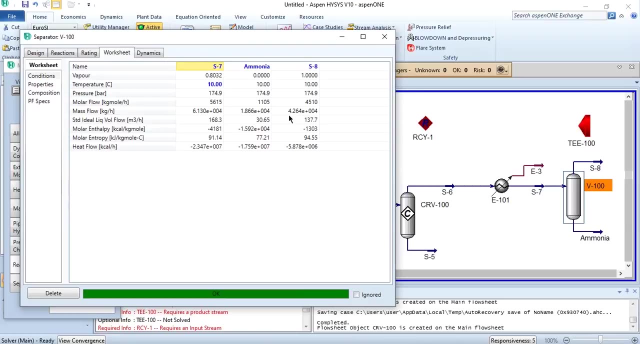 and pressure drop is 100 bar. pressure drop of 100 bar and it is 10 degrees. as you can see, not only the cooler but the separator is also solved, because the degree of freedom of separator is zero, just like the mixer. so, as you can see, ammonia is produced in the system. 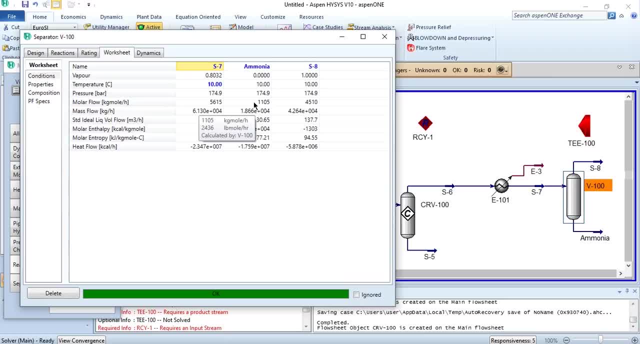 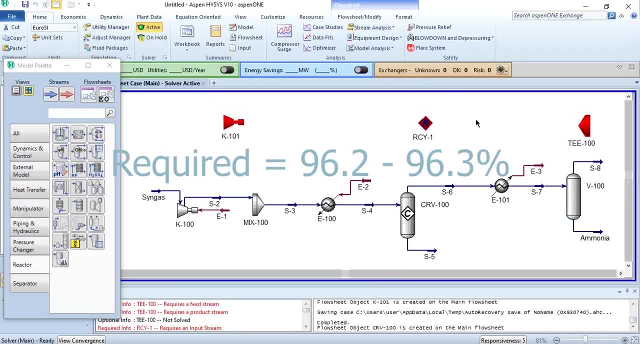 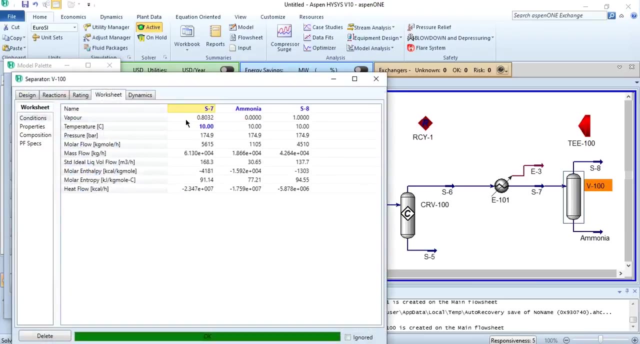 and this is the mass flow rate and this is the molar flow rate of produced ammonia in the system and the purity of ammonia is 98.06 percent. so this is the purity of ammonia before system is recycled or before this stream, which is the s8 stream. 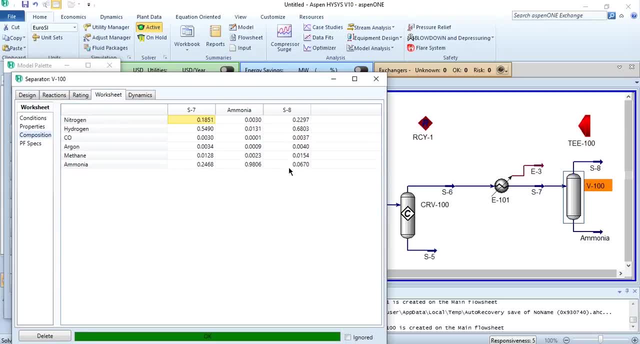 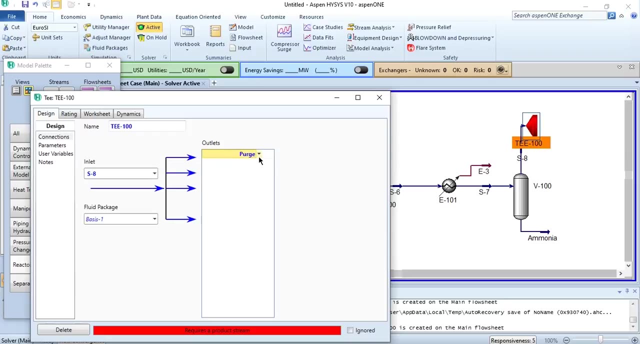 is recycled and what is the specification of a state stream? it contains ammonia, methane, argon, co hydrogen and nitrogen are also going, and some part of these are also coming from what we need to do. click on this t. the s8 stream is its inlet. one of the stream is purge and the 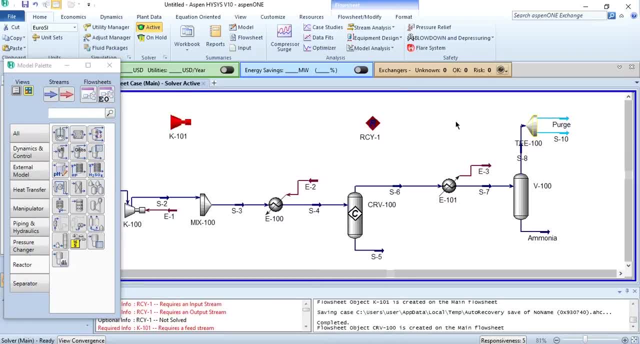 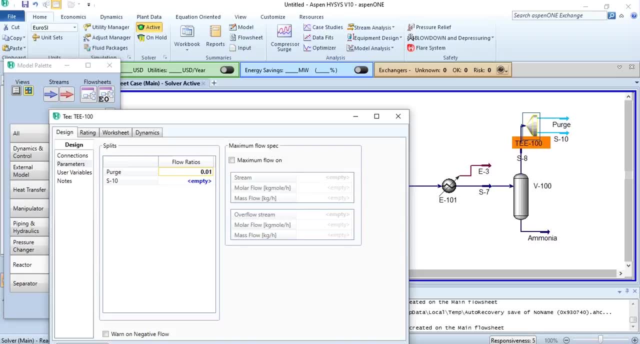 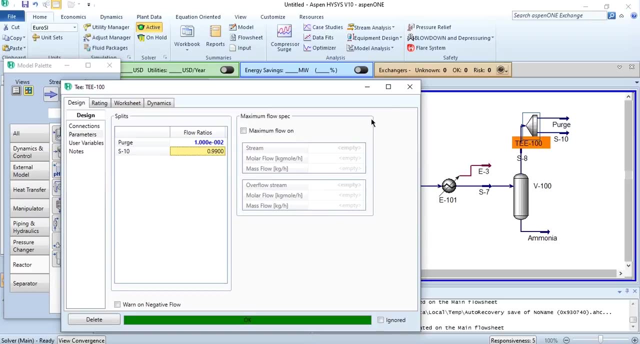 remaining stream is s 10, and if we right now give the specification of this- and what is the specification? one percent of feed stream, so it means it is 0.01. you have to specify one of these, either purge or s10. you can even specify it as 0.99, it's totally up to you, and then we can simply. 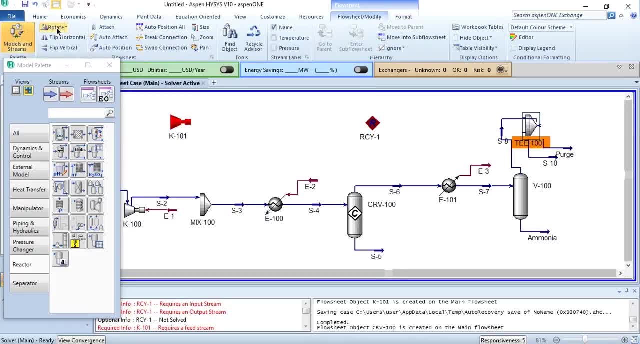 go to this flow sheet, modify, and we can click on rotate, and it will be rotated like this, if you want, like this: or it can be rotated like this: and and similarly you can put it like: and again, you can change the positions as well. so then, connected to the recycle rc by one s10. 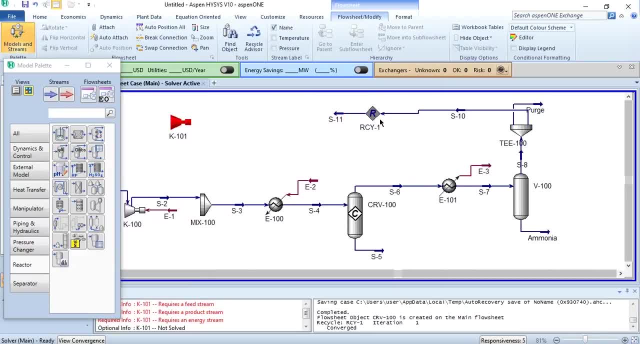 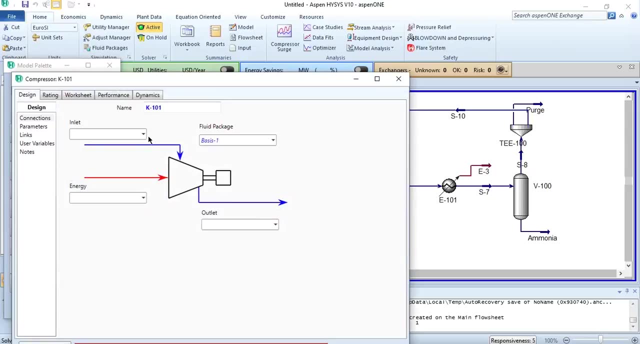 then s 11- and obviously right now it is only the recycle block- is converged, but the actual will come when it will be connected to the system, because currently it is not connected to the system. you can even rotate it as well. then s11 is entered, s12 is outlets, energy is e4. this is 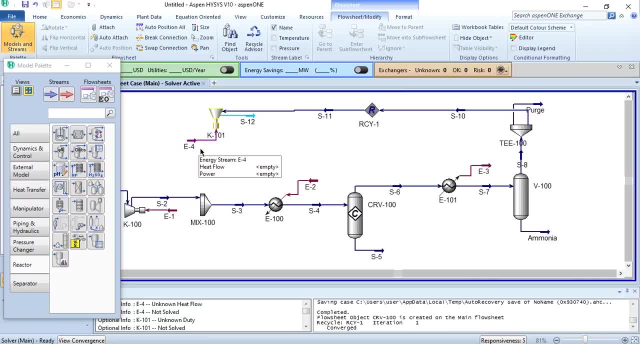 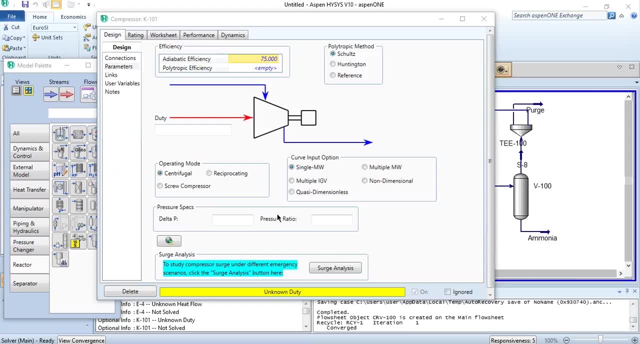 the s12 stream outlet e4 is the work required and what is the specification of it? delta p of 100.1 bar and adiabatic efficiency 75 percent. so delta p of 100.1 bar, adiabatic efficiency 75 percent. now. 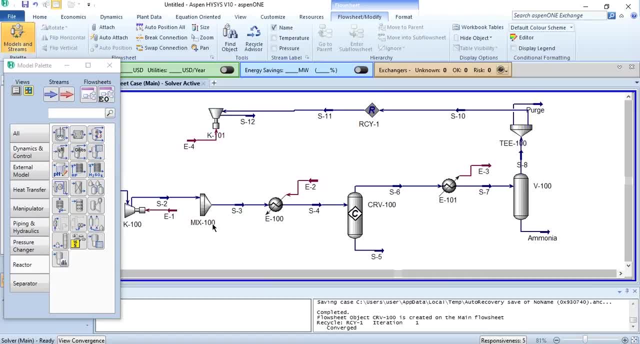 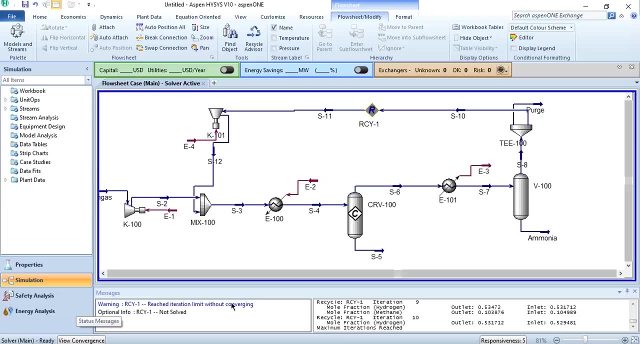 the real test will come, because now we have to connect this s12 to this mix, for which the mixer is actually installed. and this is connected and, as you can see, go to this message: warning: recycle one reached iteration limit without converging. this is currently yellow. it means that the recycle 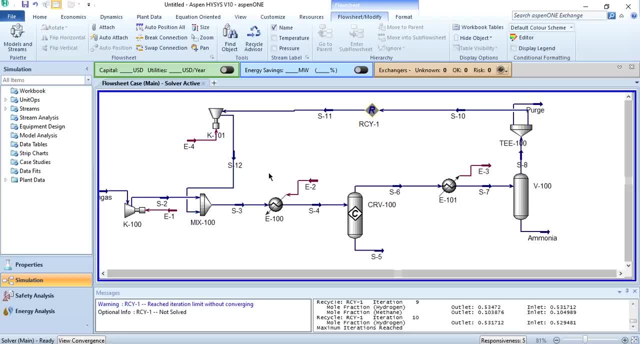 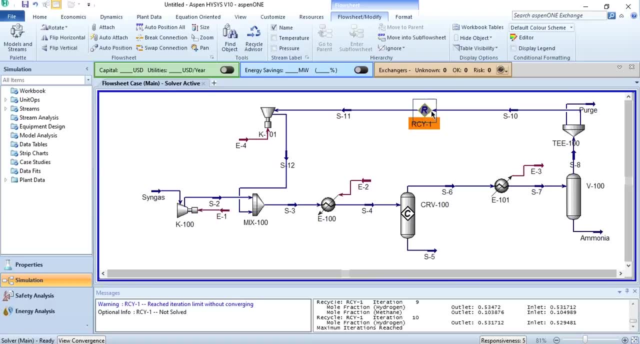 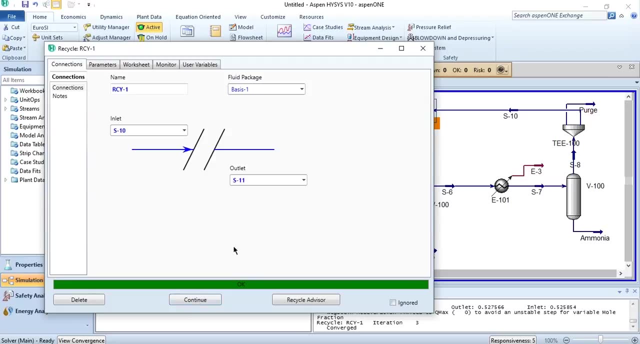 is not converged yet. it's providing you to the solution, but the solution is incomplete, and once this is incomplete, it is not correct. click on this: recycle what you need to do: continue. once you continue, this means that you have increased the iterations. so now it is converged. there is no message appearing over here. 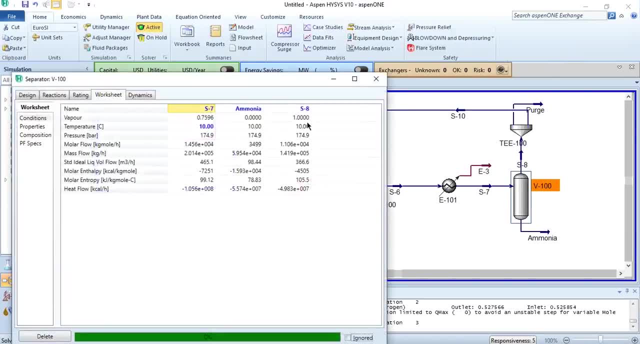 now we will see what is the improvement, and for this we go here and, as you can see, earlier it was, the molar flow rate was 1105. now the molar flow rate has increased and it is 96.2 percent, because earlier it was higher than our requirement and now it is under our requirement. 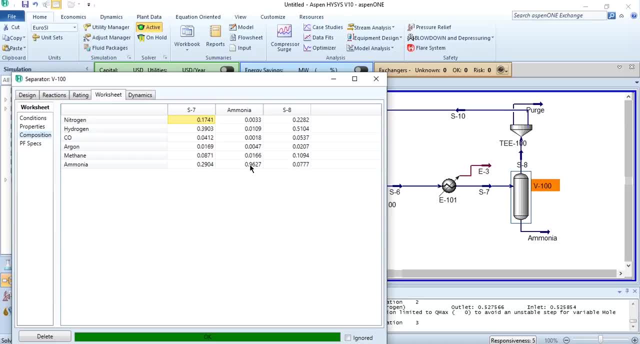 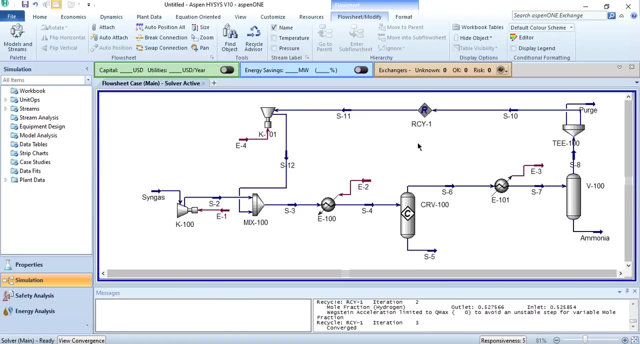 as per this design, that this design should produce somewhat about 96.2 to 96.3 percent ammonia. If you change the specification it will provide some different results. So that's how the ammonia plant is simulated in aspen ices. Currently we have used the conversion reactor. you can even 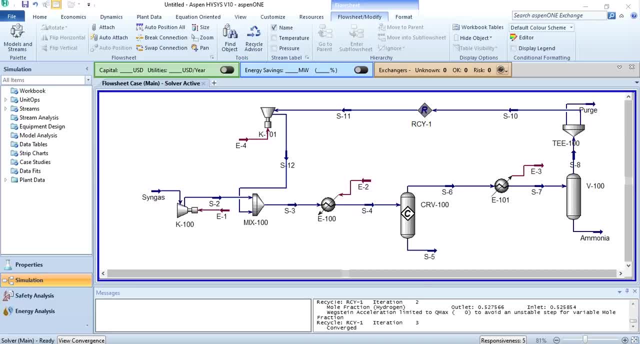 use the rigorous reactor to solve this activity. So that's it from today's activity. Please do watch, like and share the video and subscribe to the channel aspen tech. Till then, it's goodbye. stay tuned. 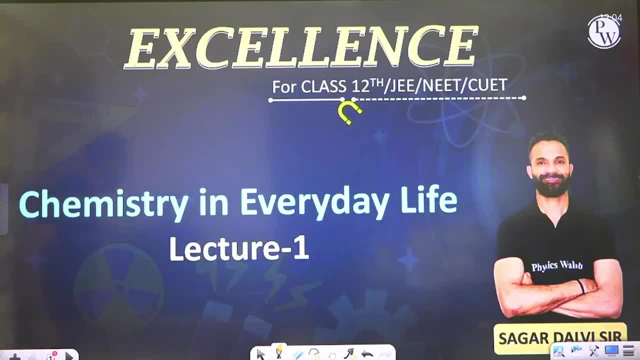 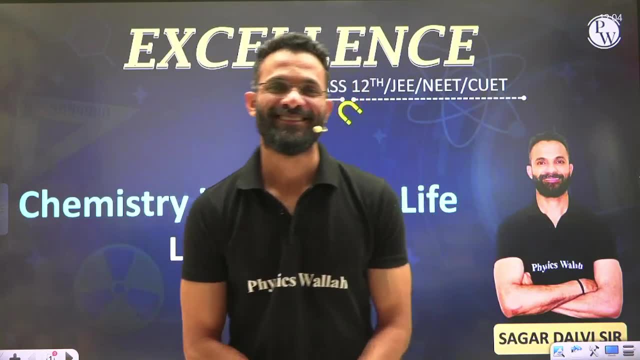 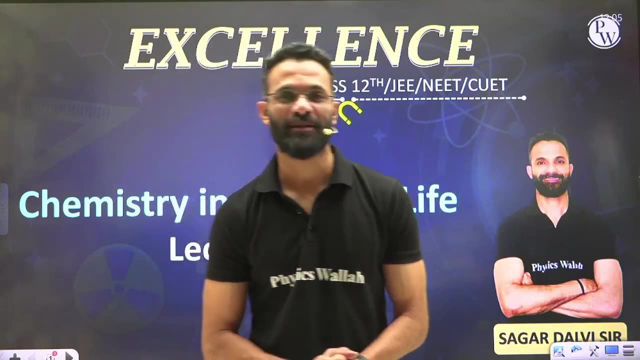 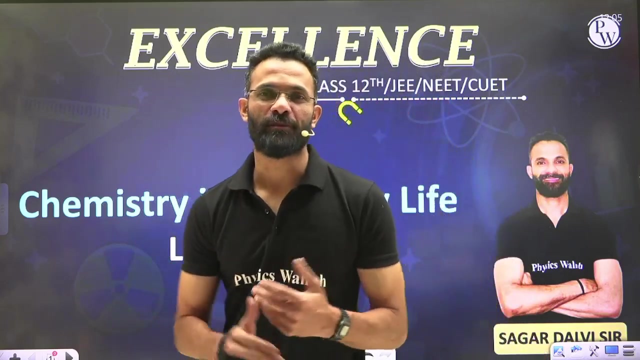 Hello everyone, welcome back to Batch of Excellence. This is Sagar Darvi, your chemistry teacher, And today we are going to discuss a new chapter, and the last chapter of organic chemistry, that is, chemistry in everyday life. Well, dear students, before we actually start with this chapter,